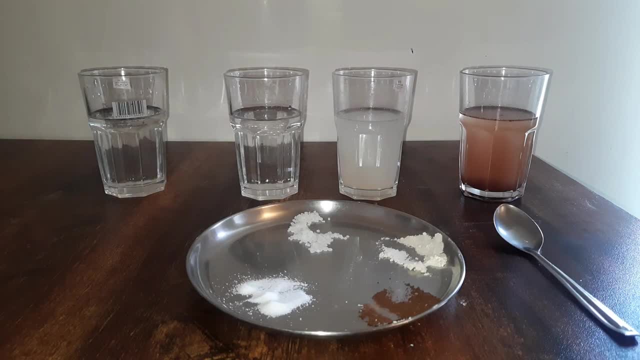 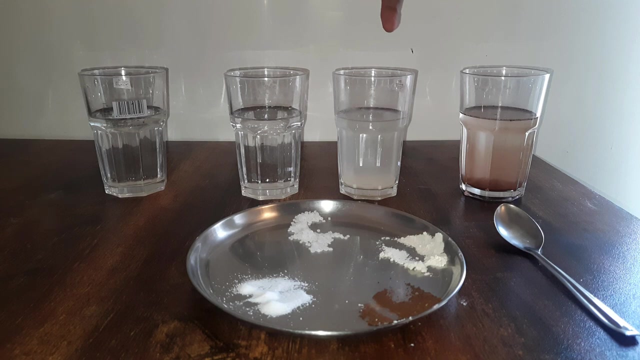 All right. so these four have now become mixtures. A mixture has two or more than two substances in it, And the first one has salt and water, This one has sugar and water, This one has flour and water, And this one has sand and water. 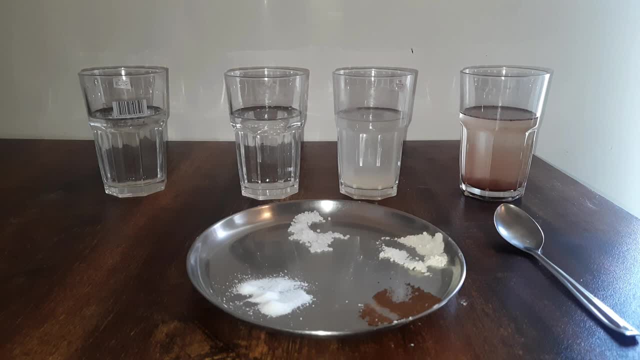 So all of these are mixtures, But I'm sure you observe some difference among them, right? Not every mixture is looking the same. Let's try and look closely. This is a mixture of salt and water. Well, are we able to see the salt that we try to mix in it? 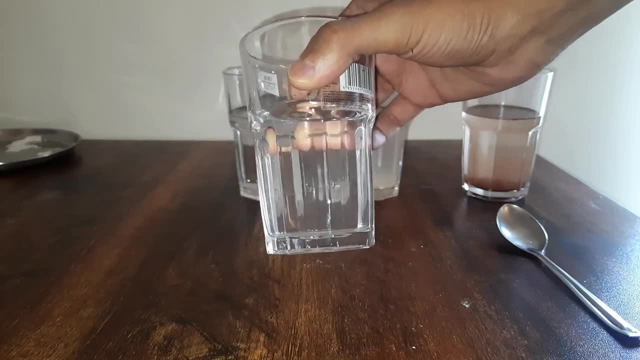 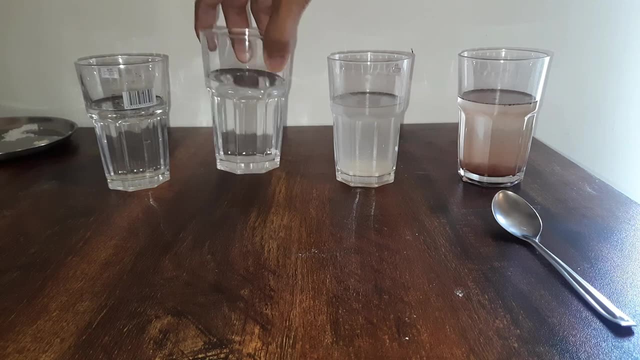 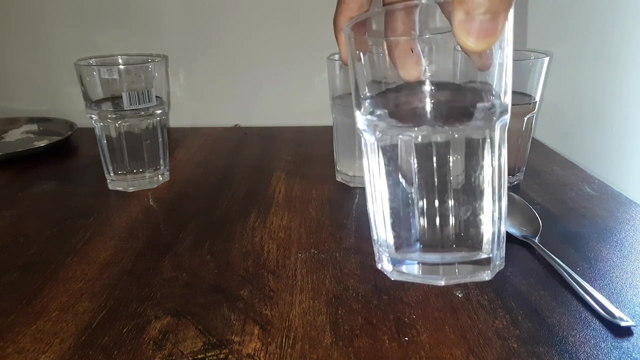 No, right, We can't see it, It's completely disappeared. Let's look at the second mixture now, that is, sugar and water. Well, again, we can't see sugar. right, It's completely dissolved, It's completely mixed with water. 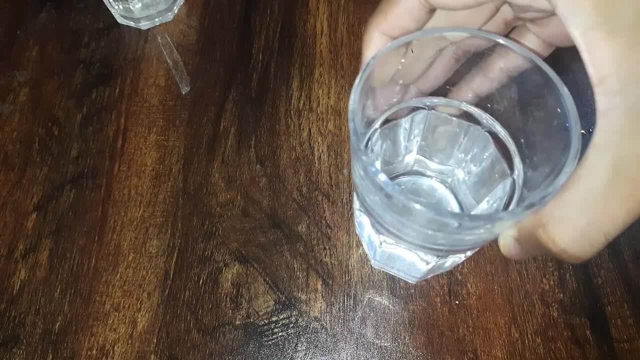 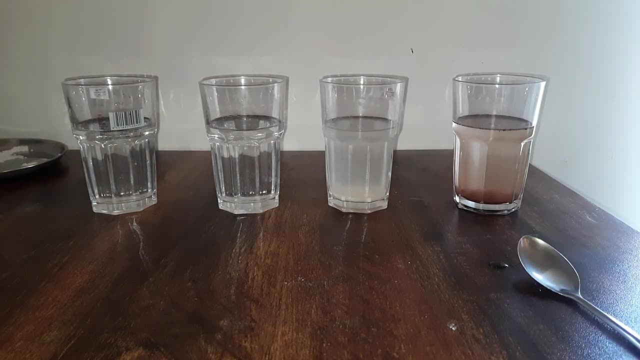 There is a little bit of left at the bottom, but you can try to mix it some more, Then gradually it will dissolve completely. So one thing is common in both of these mixtures: salt and water and sugar and water, That is, we cannot see the salt or sugar that we added to the water. 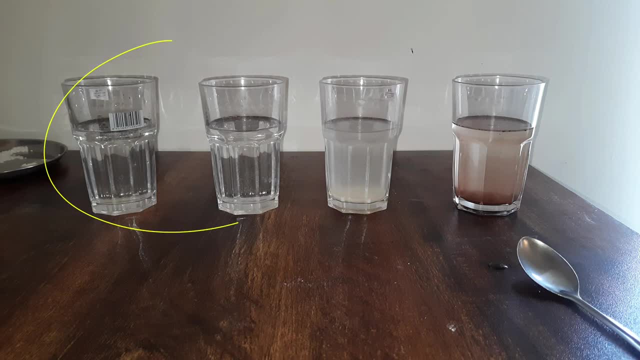 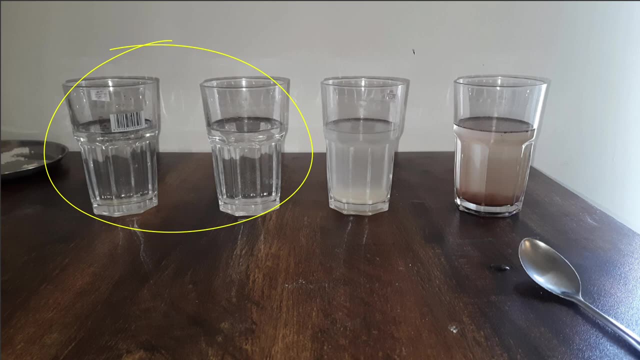 And these type of mixtures in which the components are dissolved completely, they are mixed completely, they cannot be seen- are called homogeneous mixtures. Now let's have a look at the other two mixtures. So this is the one with flour and water. 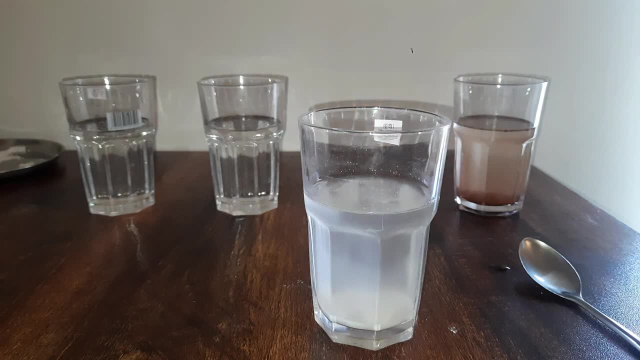 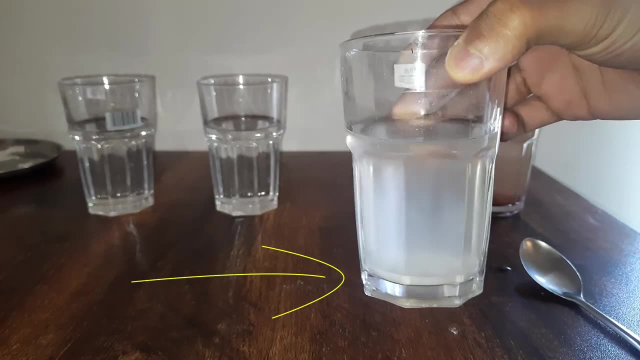 When we try to mix atta with water. Well, what do we see here? We can clearly see the flour added right. It has not Been mixed, It has not been dissolved. In fact, it has settled at the bottom. 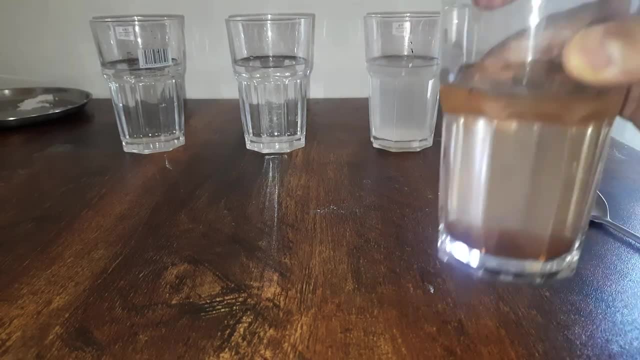 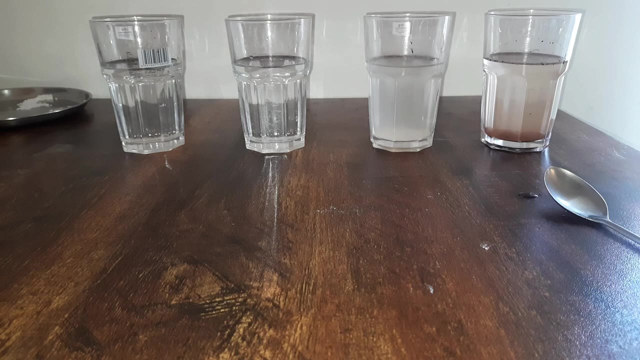 Okay, Let's look at the last mixture. Similar thing over here. right, The sand has settled at the bottom. sand did not dissolve in water. So these type of mixtures in which the components do not completely mix and the competence can be clearly seen. 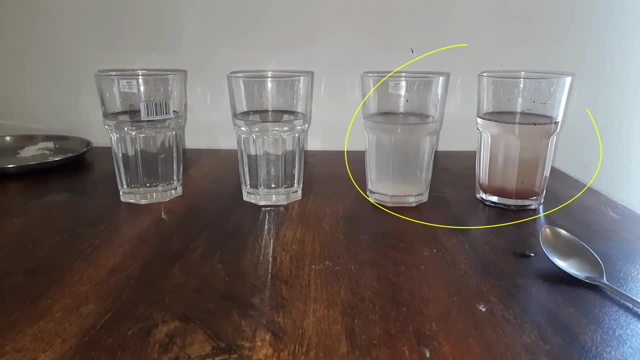 For example, we can see the flour and sand clearly in that mixture. These type of mixtures are called Heterogeneous mixtures, And there are many more examples of homogeneous and heterogeneous mixtures. Why don't you try and identify some of those examples around you? 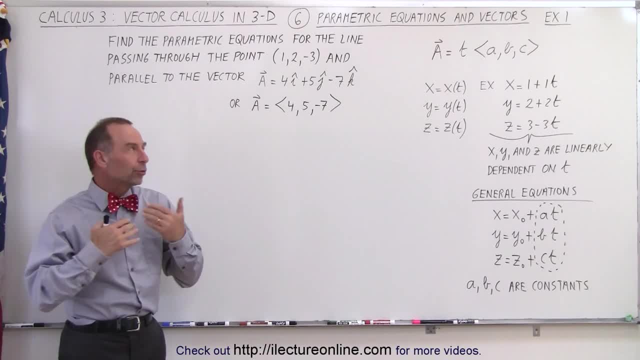 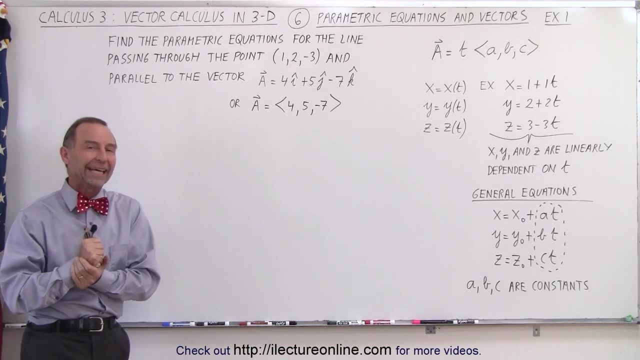 Welcome to our lecture online. Here we're going to do a simple example, but that example really helps us understand the relationship between parametric equations and vectors in three dimensions. So here the question says: find the parametric equations for the line passing through. 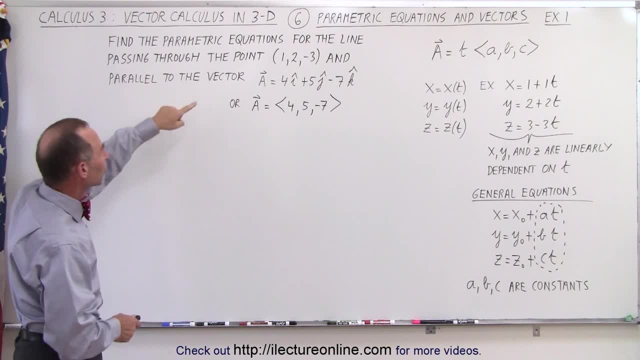 the point 1, 2, negative 3 and parallel to the vector a defined as 4i plus 5j minus 7k. So what we need to realize here is that a vector which can be written, of course, in this format. 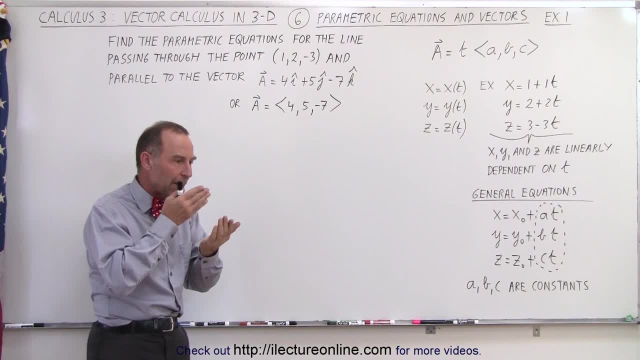 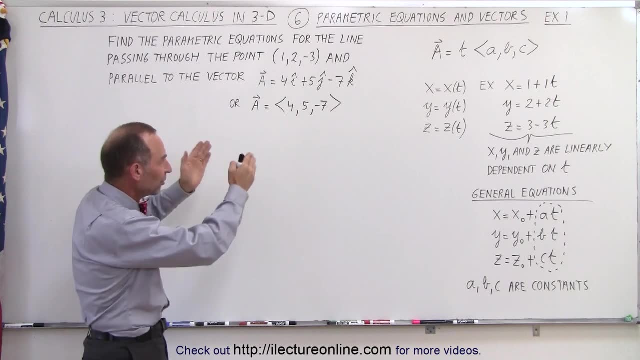 4, 5 and negative 7 are basically the amount of the change in the variables x, y and z. when there's a change in the parametric variable t, Even though it's not specifically stated, these really represent the slopes of the change in x, y and z if there's some singular change. 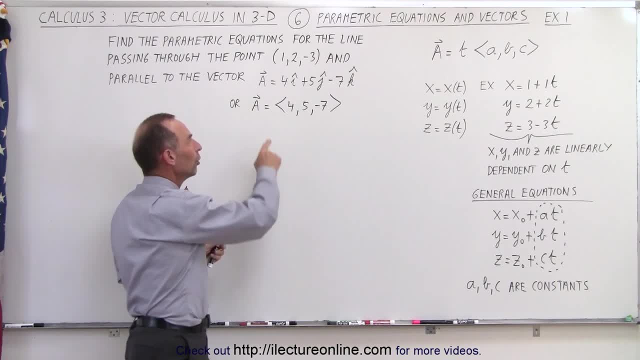 in some parametric variable driving that change. So the vector really represents how fast x, y and z will be changing relative to one another. So when x changes by 4, y will change by 5 and z will change by negative 7.. 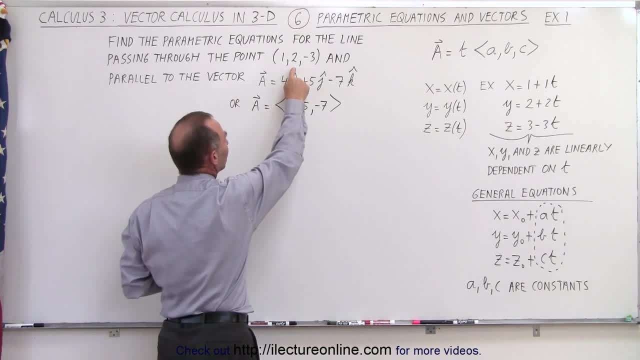 In addition to that, we're given some point that the line passes through That can be defined as some initial point, some starting point. So if that's some starting point, some initial x, some initial y and some initial z position, and then we know how much it changes. 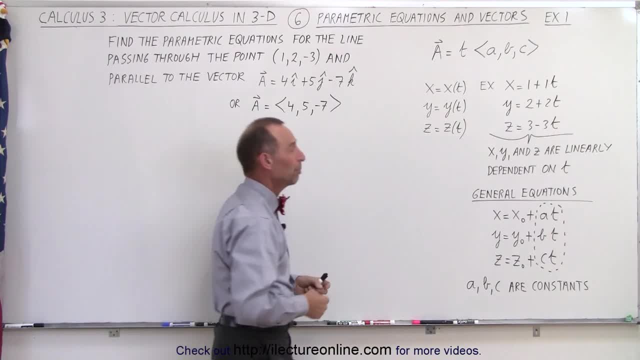 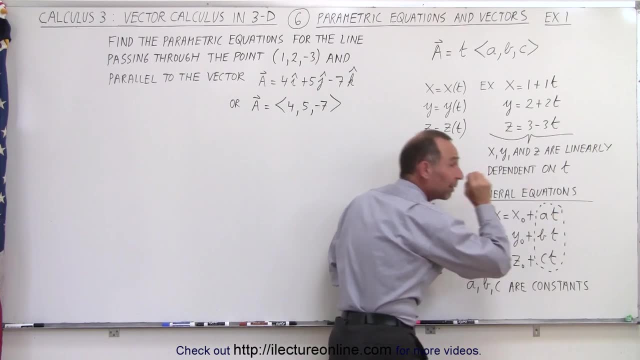 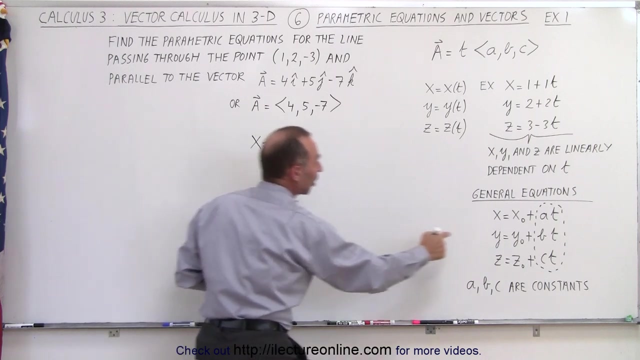 That's all we need to set up the parametric equations, because the parametric equations are defined as some initial point, plus how fast they're changing when some external parametric variable changes. So let's go ahead now and write these variables. So we have: x is equal to some.